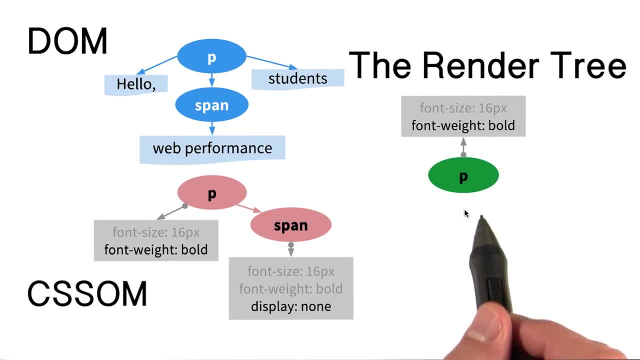 properties. Okay, we're done with the paragraph node. Let's walk down the tree. Next we see hello, which is just a text node, So we copy that to our render tree. Next we arrive at the span node. We have a matching CSS rule for it. 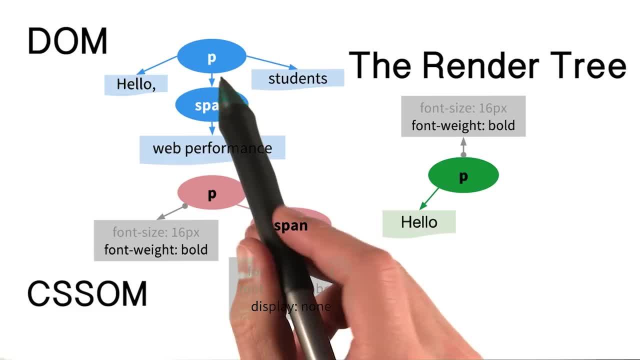 We have a span, and it is indeed a child of the paragraph node, But notice that one of the properties in this rule is that it's marked as display none, Which tells us that the contents of the span should not be rendered. And since, as we said, the render tree only captures visible content, 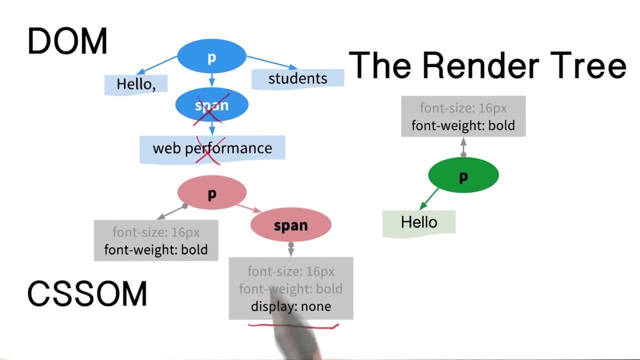 we can skip it and it's children. We skip the children because display none cascades down right Exactly And, as a result, we can skip all the children nodes of the span node and go to the next node, which, in this case, is just another text node. 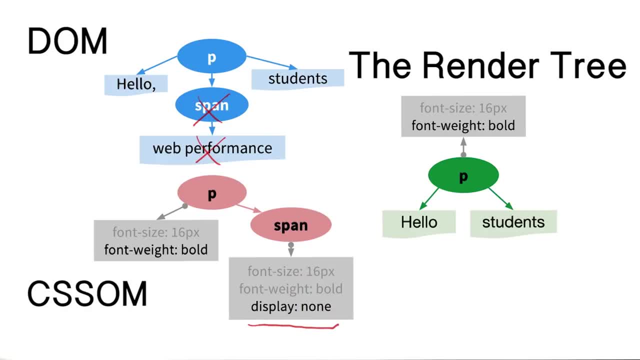 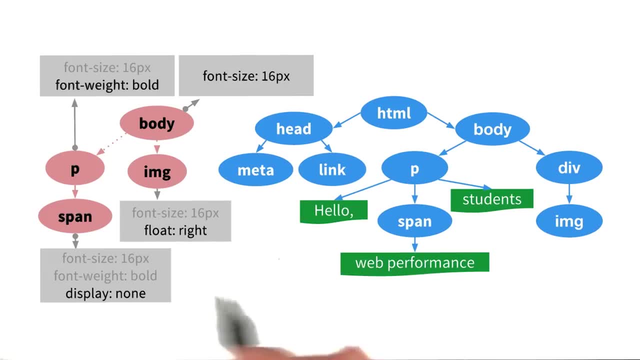 And we copy that to our our render tree once over. So the render tree captures both the content and the styles. Right Now let's take a look at our Hello World page. Okay, here we have the DOM and CSS OM trees for our Hello World page. 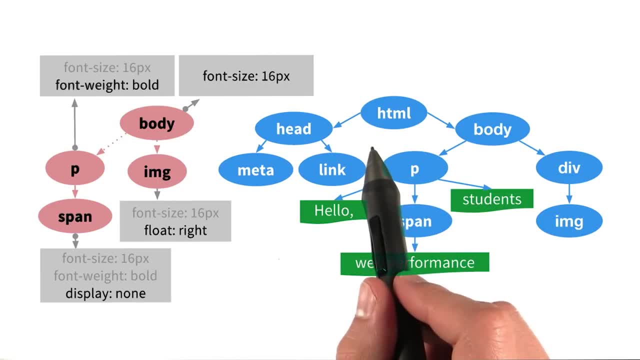 To build a render tree, we start at the HTML node in the DOM tree. The HTML and the head sections don't contain any visible information, So we can just quickly prune them out of our render tree. Next we have the body node. 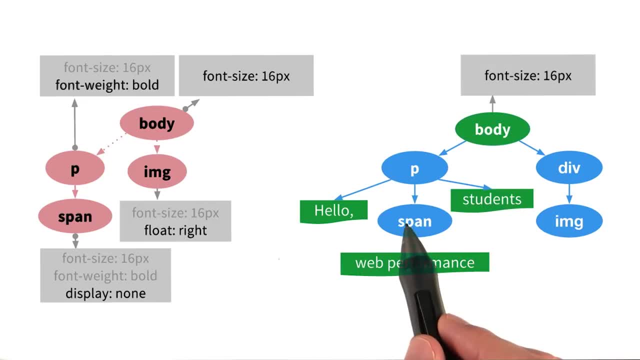 Let's copy that over. This left part of the tree should look familiar. This is what we just built, so let's copy that over as well. Finally, we have the div and the image nodes. Both of these contain visible content, so we also copy them over and. 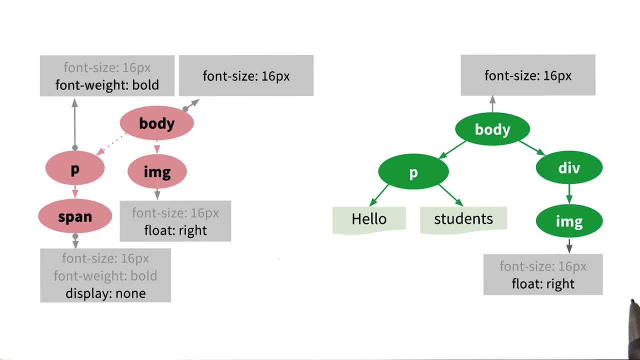 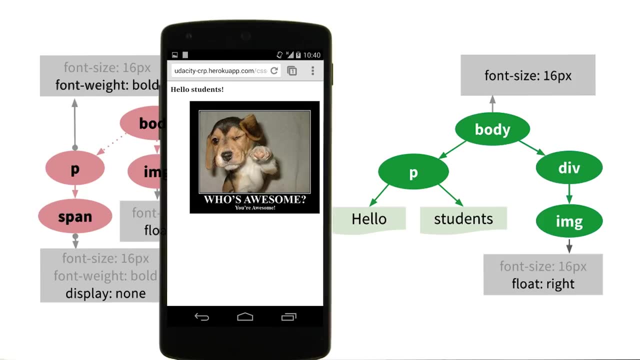 their styles into our render tree. With that done, compare this render tree to what we have on the screen. Huh, yeah, the render tree is a pretty good representation. The unnecessary text is gone. I can see that there should be an image on the screen and. 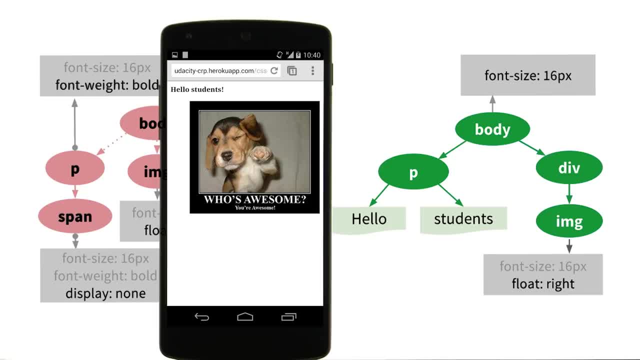 it should be displayed on the right. So are we all done now? Not quite, We still have to do layout. but first a quick quiz.